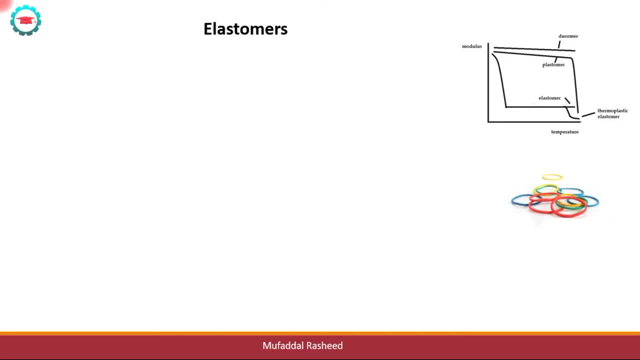 Now we will understand more about elastomers, which are a sub classification under polymers or plastics. So elastomers are a type of amorphous polymers or amorphous plastics which exhibit rubber like elasticity. So we have seen in the lecture on glass transition temperature that 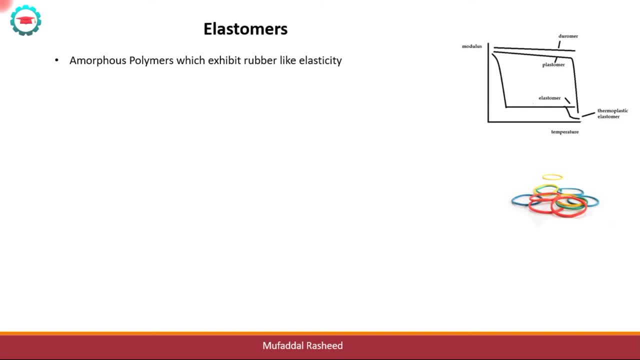 the plastics, the amorphous plastics, will transform from glassy state to rubbery state. This transformation results in the drop of the modulus and the material starts to behave viscoelastic in nature. The difference between elastic and viscoelastic behavior is shown over here. 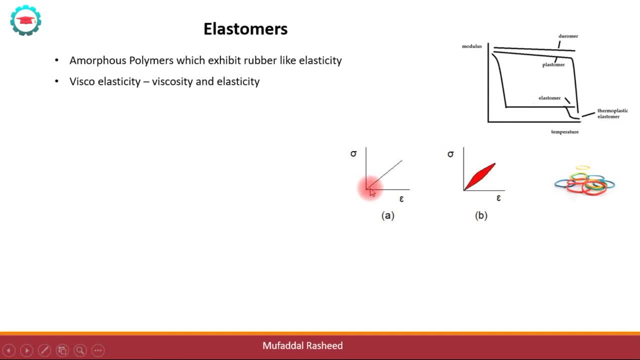 So this is elastic deformation in which the stress is directly proportional to the strain. This is viscoelastic deformation in which the stress is not directly proportional to the strain and it is a curve and also the loading and unloading cycles are not the same Over here. 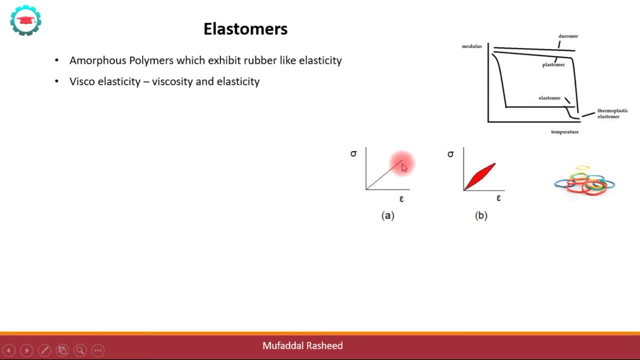 in a purely elastic deformation the loading and unloading will be on the same line. There will not be any energy ência loss. but over here there is energy loss between the loading and unloading cycle. so we have seen that in the loss coefficient. so a viscoelastic material will have higher loss coefficient. 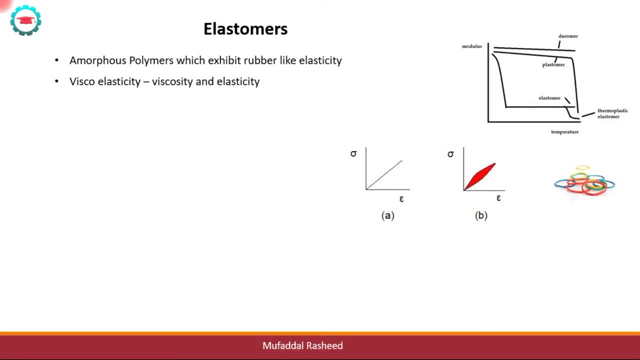 as compared to an elastic material. so this gives them the properties of low modulus and extremely high viscoelastic deformations, even at low loads. so glassy state plastics or plastics which are harder and rigid do not have such properties. but elastomers have such properties because 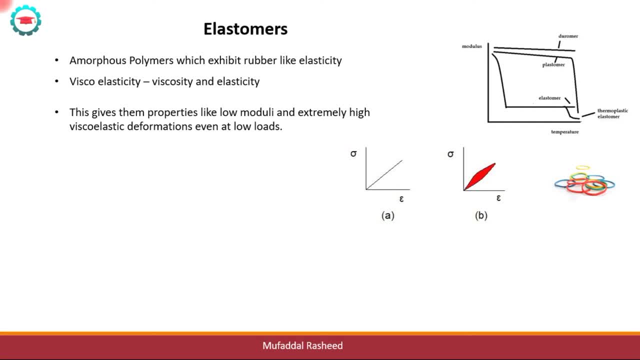 they are viscoelastic in nature. this viscoelastic nature is also called as rubbery nature, because rubber is the main material which is considered as the main elastomer which is generally used in industry. so the way rubber behaves is generally a template for other elastomers also. 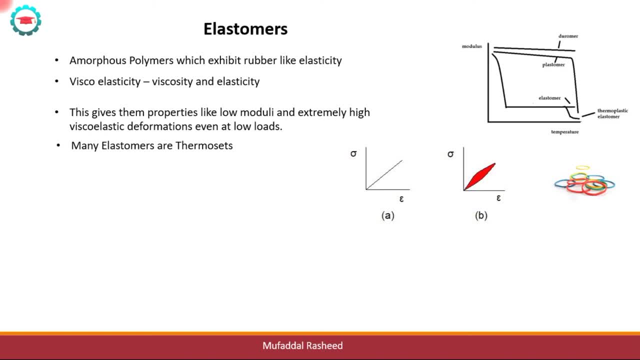 one differentiating fact of elastomers is that many elastomers are generally thermo setting plastics, which means that they are difficult to process once they have been already molded, so they cannot be melted and remolded like thermoplastics can, and hence processing waste becomes a problem. some common examples of elastomers include natural rubber, which is: 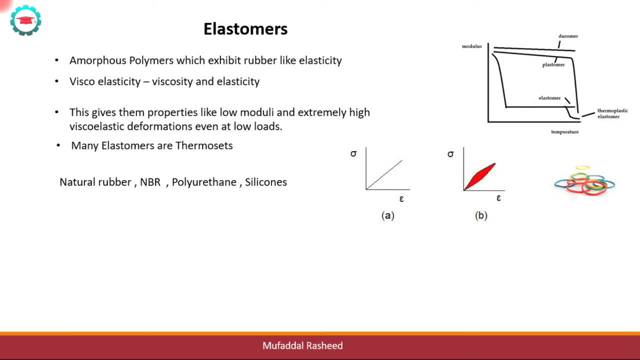 naturally occurring substance extracted from trees. nbr is a synthetic rubber which is chemically synthesized polyurethane. is can be used as an alternative to rubber, which is a highly tough and highly fracture resistant material which is commonly used in the form of bushes or mounts in automotive applications and also used as a good replacement for rubber, because it has 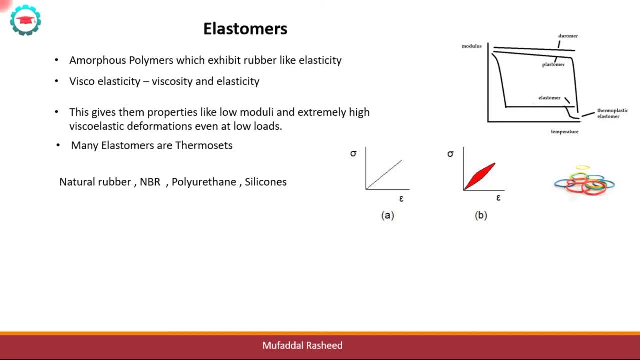 better characteristics in terms of durability. silicones are soft elastomers which are used in the manufacture of toys, in the manufacture of medical implants and many other various applications which do not require as much durability as natural rubber or polyurethane does, since they are thermo setting plastics. processing is a problem processing. 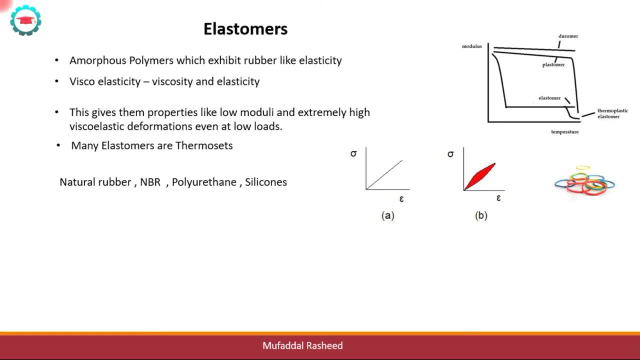 costs higher and hence elastomers are generally costlier as compared to thermoplastics- the generic thermoplastics also. they have a wide part to part deviations of properties, so if you are manufacturing a hundred parts the deviations of those properties can be high. that is a 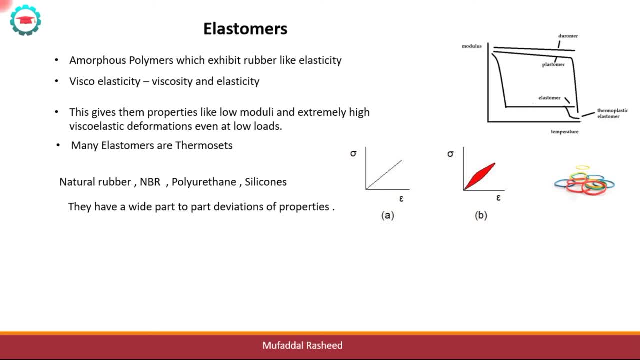 characteristic of elastomers. for example, rubber bushes, which are used in automotive applications for vibration isolation, have a very wide part to part deviations, almost to the range of plus or minus 15 percentage, that is, for plus or minus 15 percentage change in this stiffness is accommodated. 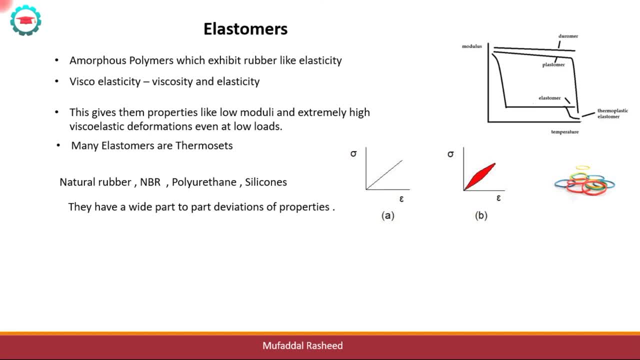 in such applications. now, if you compare elastomers to the generic polymers or thermoplastics which we have already seen, generic polymers like pp, pc, abs, nylon, these no need for airflowください. These polymers are generally hard and stiff, compared to elastomers, which are softer and 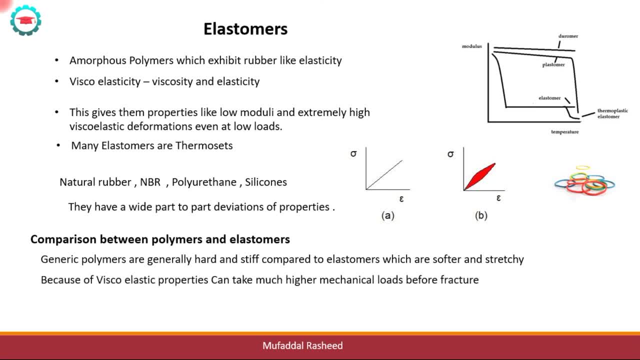 stretchier like rubber. Because of the viscoelastic properties, elastomers can take much higher mechanical loads before they undergo fracture and they have much higher internal damping properties. So this is a very important property of elastomers, which is why they are used for vibration isolation. 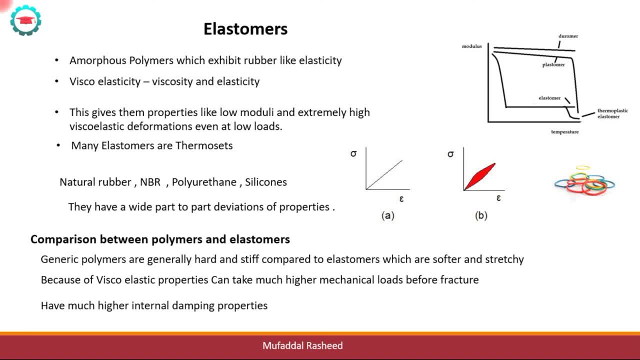 As we have seen in the lecture of loss coefficient and the damping properties, the amount of energy lost between the loading and unloading cycle will basically decide how good a damping material that is. Elastomers generally have a very high gap over here and hence lose a lot of energy between